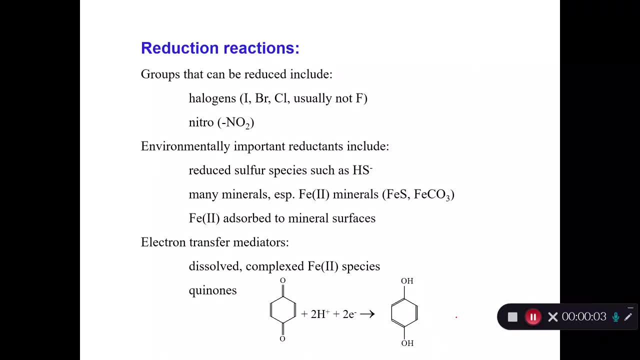 Hi everybody. Welcome back to Environmental Organic Chemistry with Dr Lisa. We're going to continue our discussion of redox reactions by talking about reduction reactions. Remember we had a very, very short, little lecture on oxidation reactions, but most of the reactions 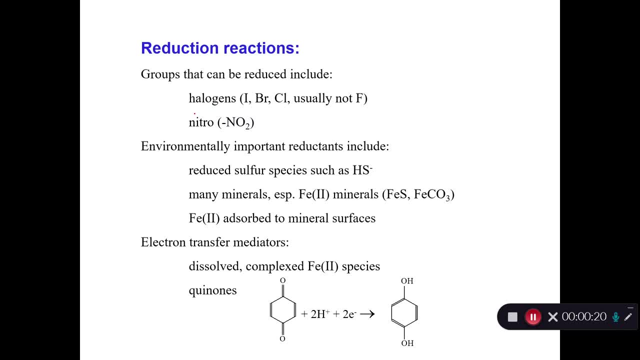 that we're interested in that occur in the environment tend to be reduction reactions, because chemicals are designed to be stable under oxidative conditions- ie out in the world where there's oxygen- But they're generally not designed to be stable under reductive conditions. So the 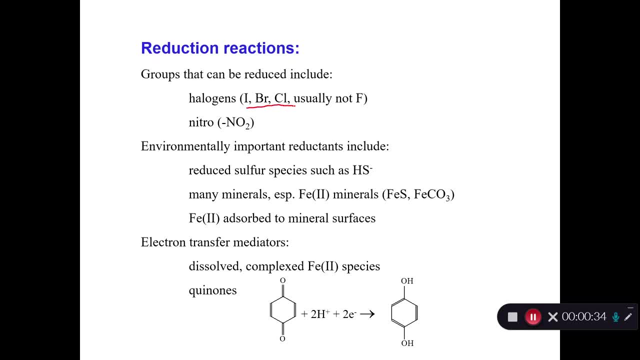 kinds of groups that can be reduced are any of the halogens, iodide bromide chloride, And here I've said usually not fluoride. but we have some evidence now for the defluorination of PFAS, which I'll talk about at the end of this, not the end of this video, but at the end of another one. 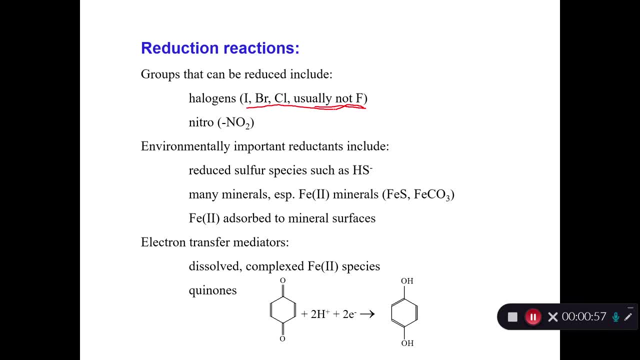 later on. So removal of fluorine is not as common but it does sometimes happen. But definitely iodide bromide and chloride can be reductively removed. Nitro groups again also can be reduced down to aniline-type groups or amines And the types of things that act as reductants. 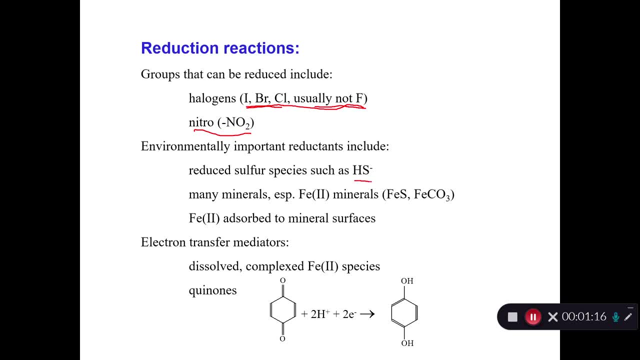 that provide the electrons to make this happen are things like reduced sulfur species, iron-2 minerals, iron-2 sorbed mineral surfaces, iron-2 porphyrins, which is what I mean here by complex iron-2 species, and our friends, the quinolones that we saw before. 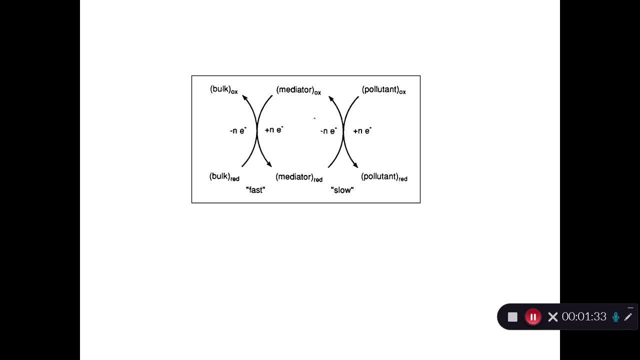 So remember we also talked about this- the fact that our chemical- here here's our pollutant- is usually in an oxidated oxid, oxid, meh high oxidation state, and it gets reduced. So here's the high oxidation state pollutant and here's the reduced pollutant. And to do that somebody has to. 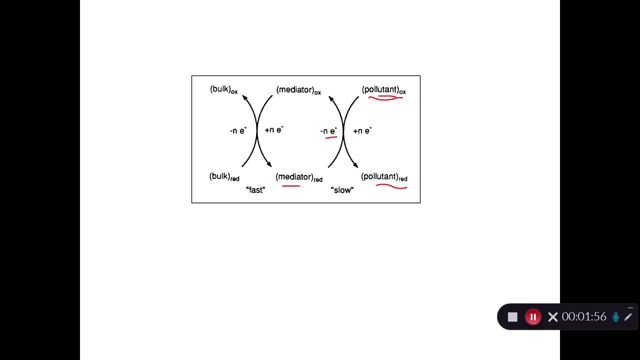 donate some electrons and then you can see that there's a lot of cyanide and there's a lot of Those electrons frequently come from some sort of mediator in the environment that donates its electrons, goes from a reduced mediator to an oxidized mediator and then the oxidized 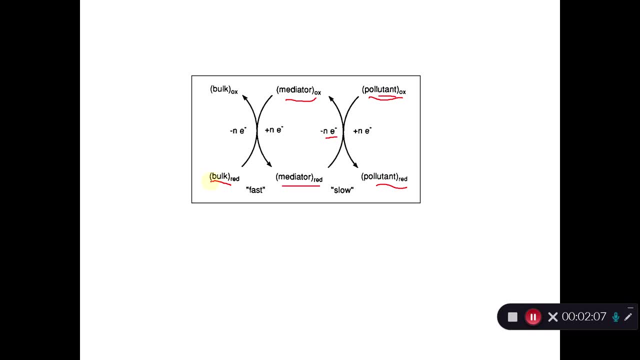 mediator reacts with some bulk source of electrons- which again could be surfaces or something like that- that give up its electrons. so the surface is getting oxidized, But the pollutant generally doesn't react directly with the bulk donor because of mass transfer limitations and other things. 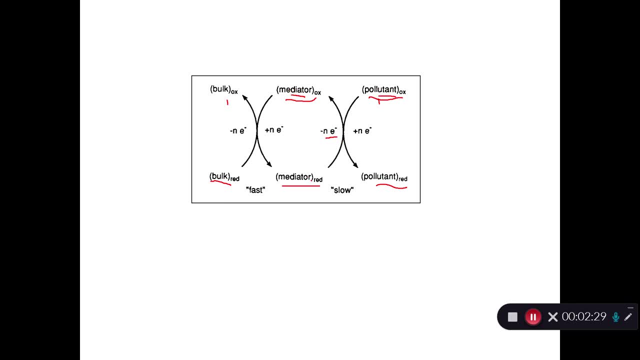 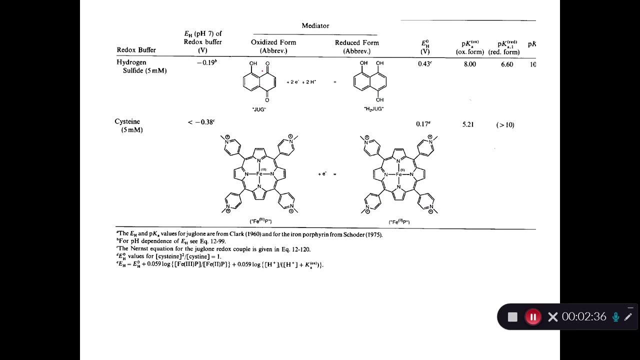 It's more common that the pollutant will react with some sort of mediator that shuttles electrons around through our system, And we have already discussed the fact that there are these quinones that act as electron shuttles that move electrons back and forth, because this is a very reversible chemical. 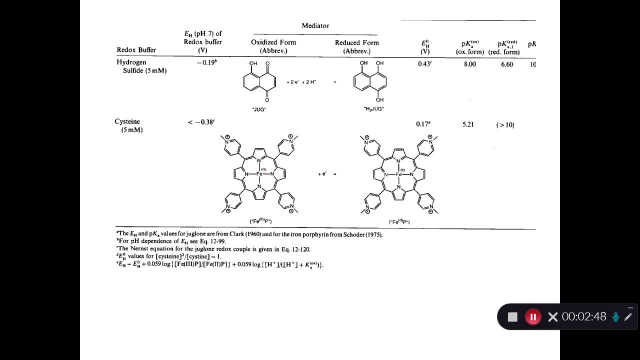 reaction. And then here's an example of our iron-2 porphyrin: here's iron-3 and here it's in the iron-2 form, so it shuttles electrons back and forth. There's a pKa involved, because there's exchangeable protons here. 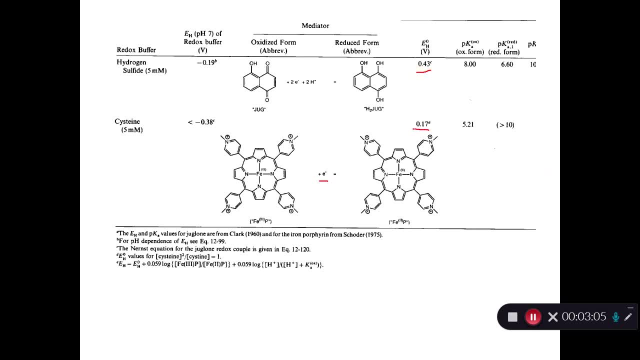 But here's the redox potentials and you know they're positive and reasonably favorable. So these things make good redox shuttles. Also, I don't really like the way that this is organized, but here's hydrogen sulfide and then here's cysteine, which is an amino acid. it also has a favorable redox potential. 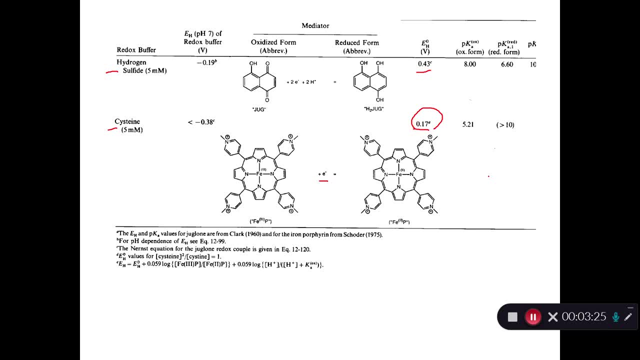 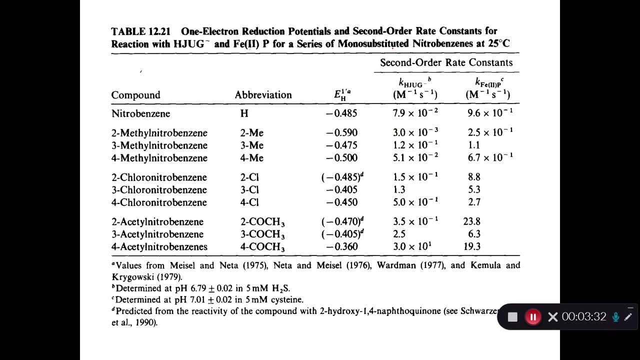 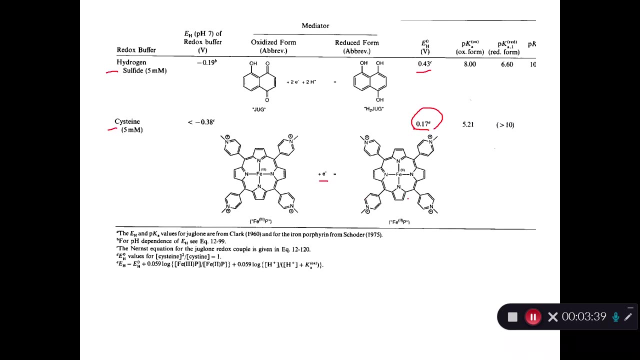 And then the iron-2.. porphyrin is shown here, but it doesn't really have a redox potential given. So here's a table of one-electron reduction potentials and second-order rate constants for the reactions of this: juglone, that's this thing, and iron-2 porphyrin, that's this. 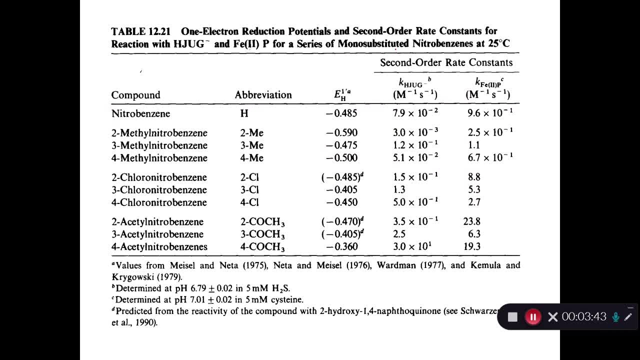 thing with a series of substituted nitrobenzines at 25 degrees C. Okay, so they all have the nitrobenzene structure, but then, attached to the nitrobenzene, they have in this case some methyl groups. 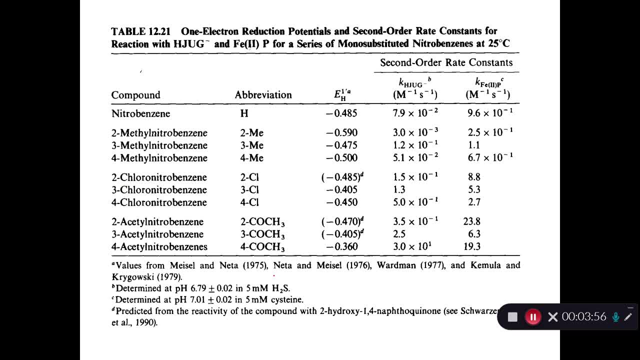 Or a chlorine or an acetyl group, And they are substituted at the different two, three and four positions. And then here's the redox potentials that they've measured and the rate constants for reactions with juglone and reactions with iron-2 porphyrin. 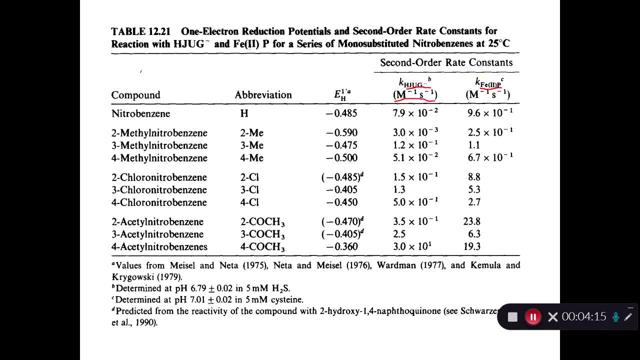 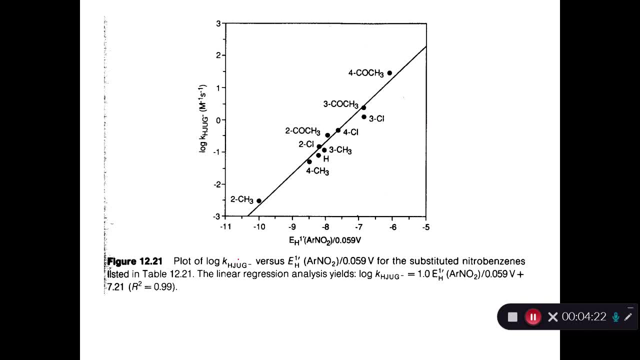 Notice that these are second-order rate constants and you know that by looking at the units per molar per second. And if you plot these, you look at something like this. So here's your redox potential and here's your rate constant. log of your rate constant.